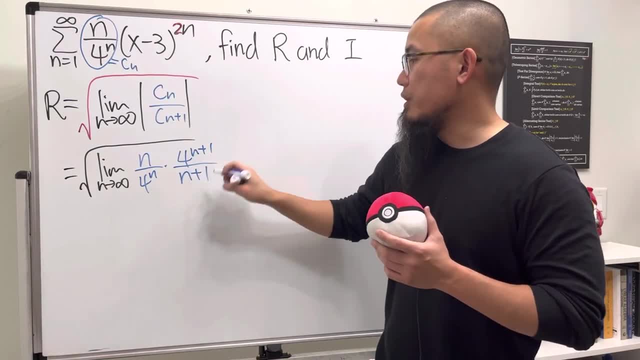 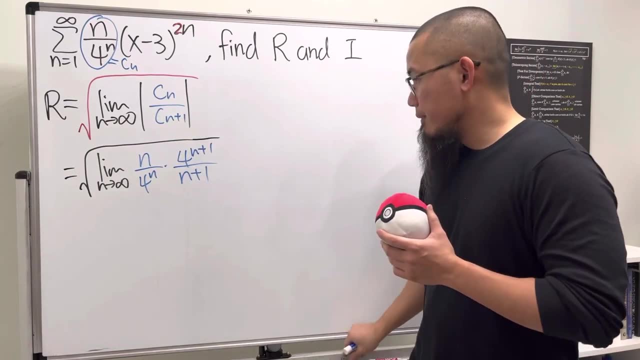 here, and likewise I'll put that down on the bottom with n plus 1 here, And the absolute value doesn't matter because everything is positive inside. so that's good. And we see: 4 to the n plus 1 can be written as 4 to the n times 4 to the n. 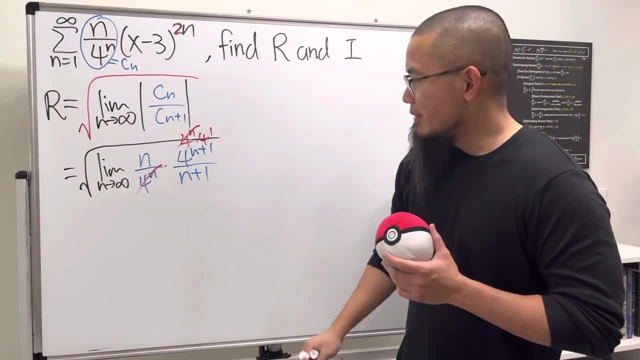 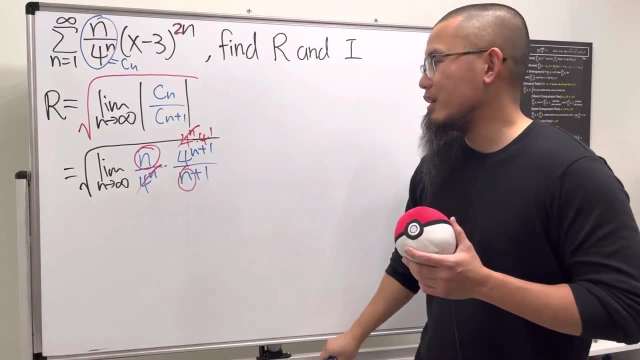 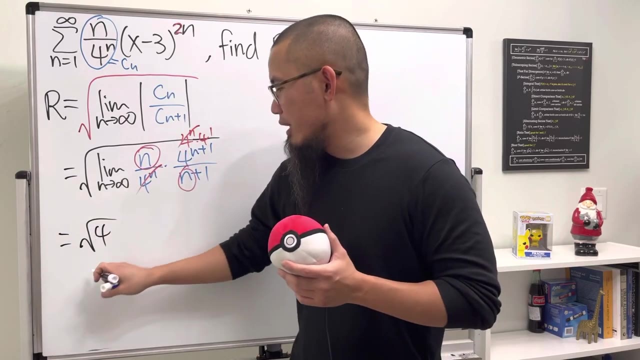 And this and that, cancel Nice. And then, as n goes to infinity, we just care about n and we just care about n. right here, The plus 1 doesn't matter. So just work out the limit real quick. You will get square root and everything inside is 4.. And, of course, take the square root of that. it's just. 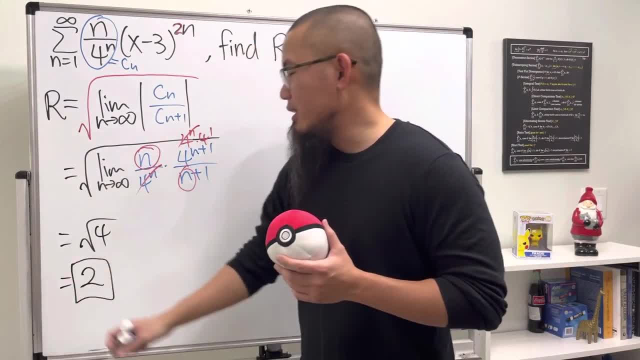 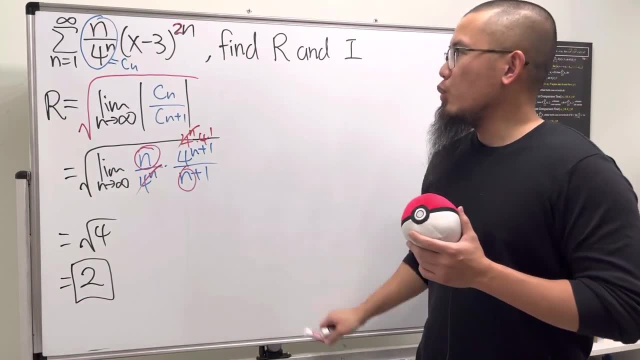 2.. So there we have it. r is just nice. d equal to 2.. Now take a look right here. This is the power of r. So in order to find out the interval of convergence, not only we need to know the radius. 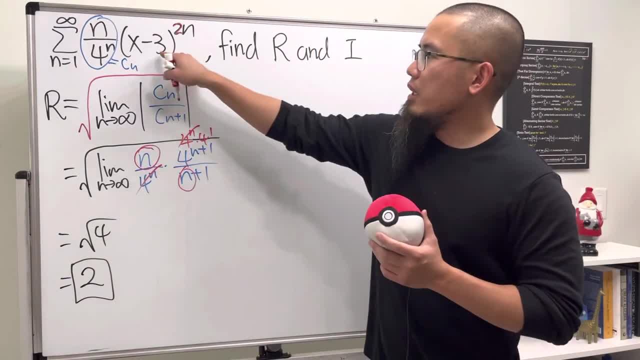 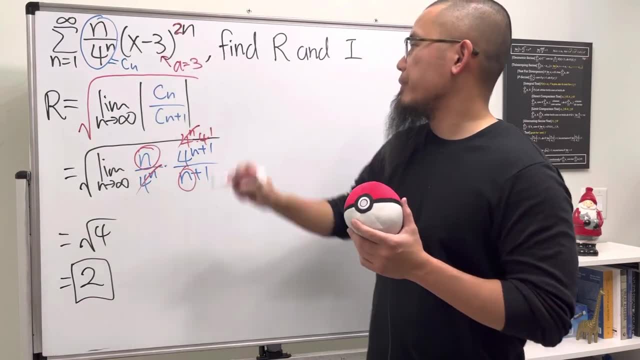 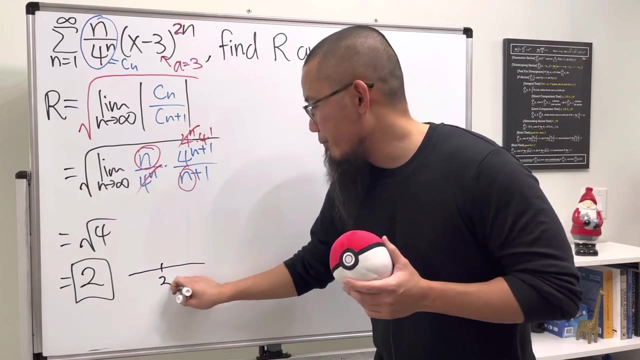 of convergence, but also the center. Here is the center. We have x minus a, a is 3.. So a is equal to 3.. This means the following: We have the number line and the 3 is right here, And of course, 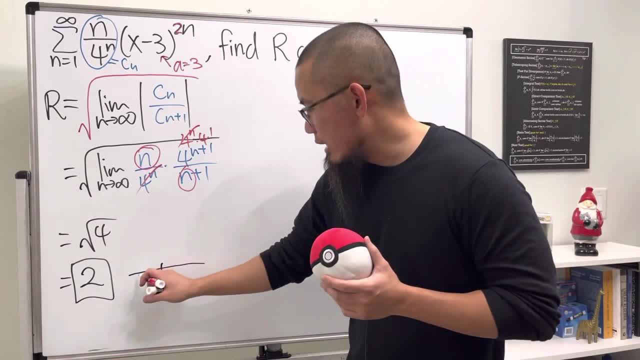 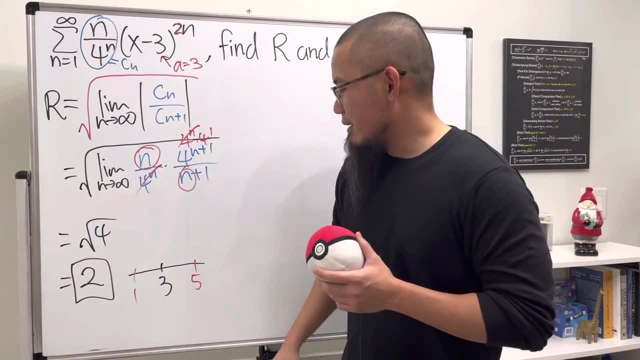 the radius means that we can go to the left and go to the right. So if you move to the left two times, we get 1.. And if you move it to the right twice, you get 5.. So again 2 this way and then 2 this way. 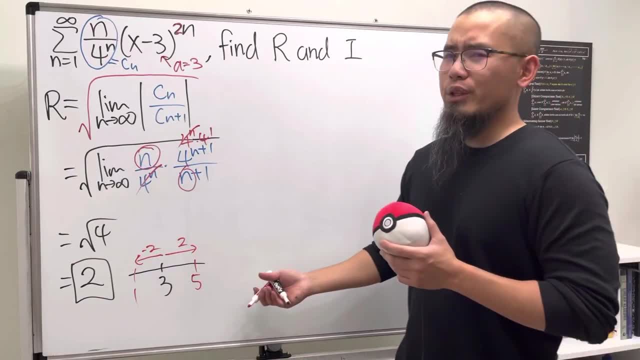 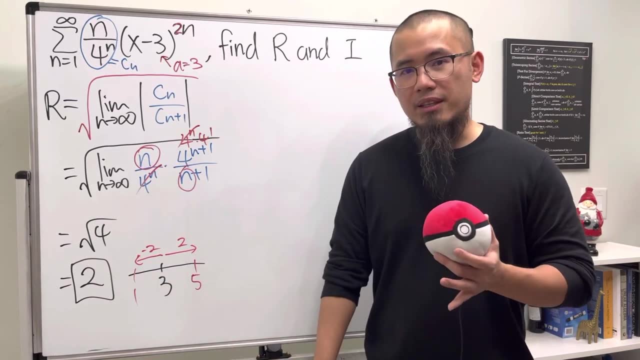 Minus 2 and plus 2, pretty much. And you might be wondering why is this called the radius? Because we are only going left and right. The reason is because this is one-dimensional. Later on, if you ever take a complex analysis course, you will see that when we are talking about a 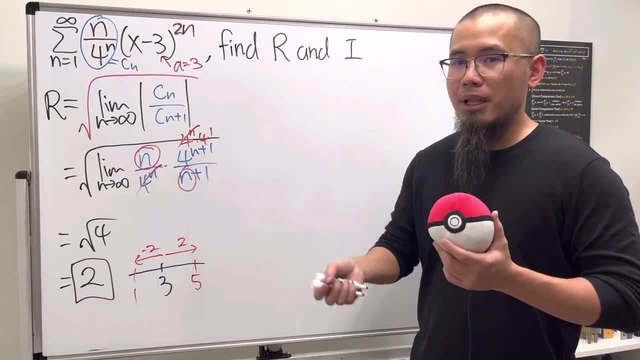 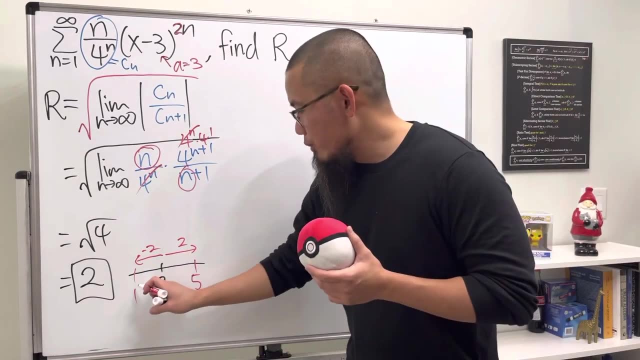 two-dimensional case, like x and y plane It is. It's really a circle. That's why it's the radius of convergence. But anyway, we do not know what will happen when x is equal to 1.. We do not know what will happen when x is equal to 5.. So you must. 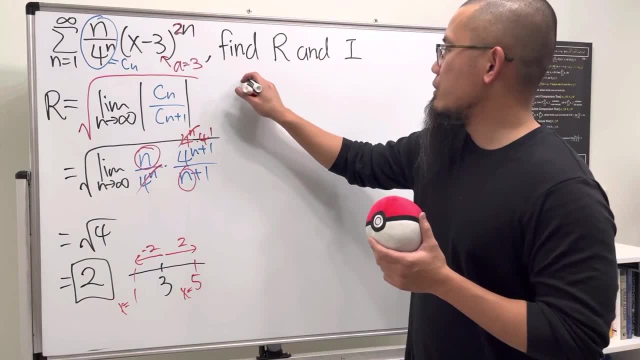 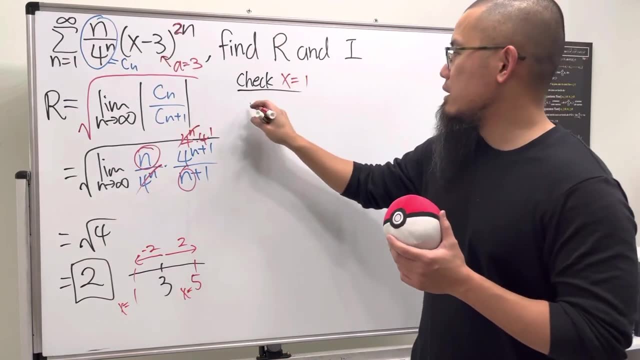 test it out. So here we go. We are going to check When x is equal to 1, let's just go ahead and put a 1 in here and we will get the series As n goes from 1 to infinity, n over 4 to the n. 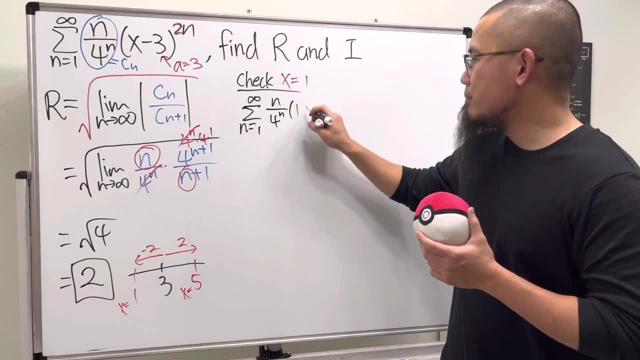 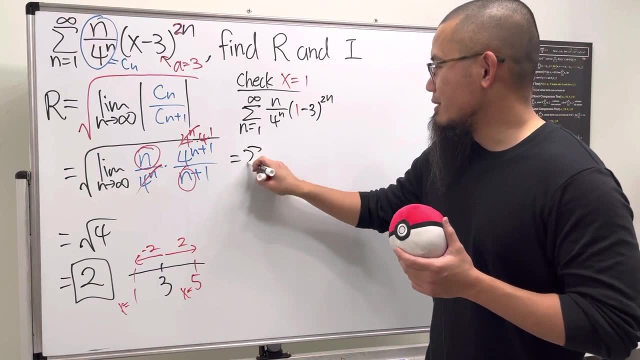 negative. so let me show you guys the work: 1 minus 3. and then to the 2n's power. inside here we get negative 2. so here this is the series, as n goes from 1 to infinity and over 4 to the n, and then 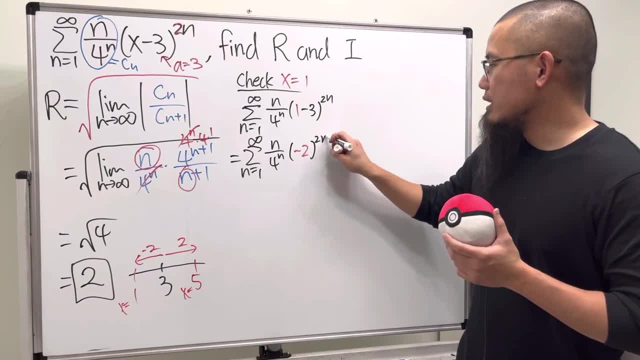 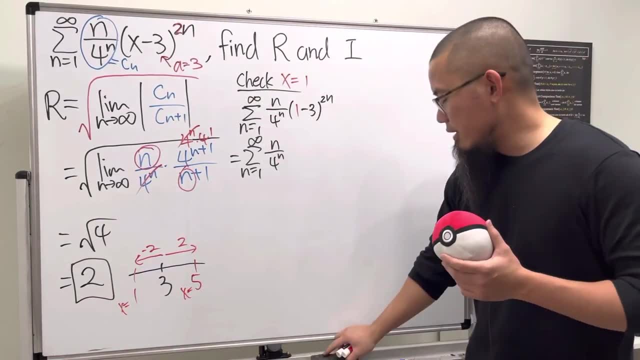 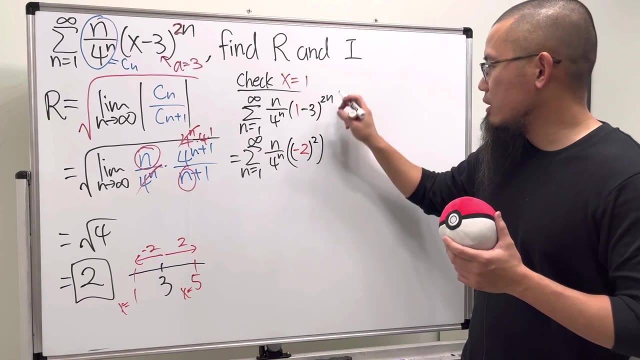 we have the negative 2 raised to the 2n's power. but for this right here, what we can do is we can actually do the second power first and then the n's power. so this right here it's a negative 2, and then let's do the second power and then let's do the n's power. so in fact, this right here is: 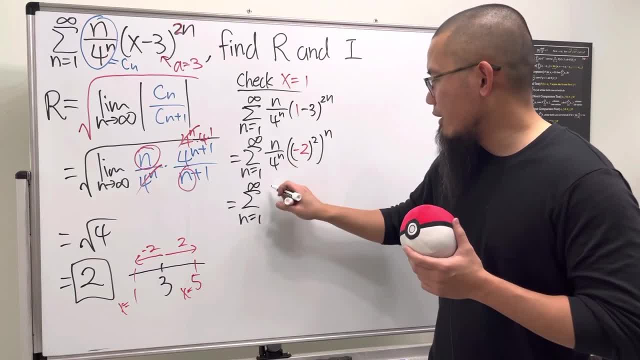 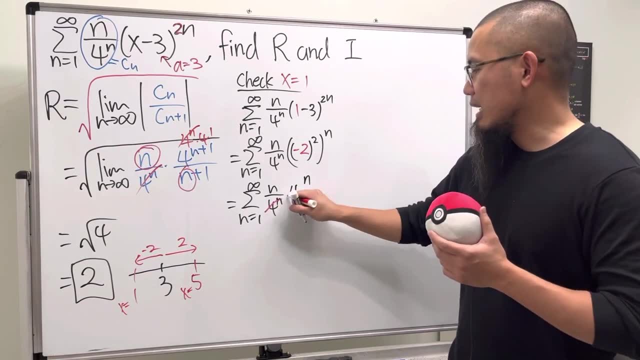 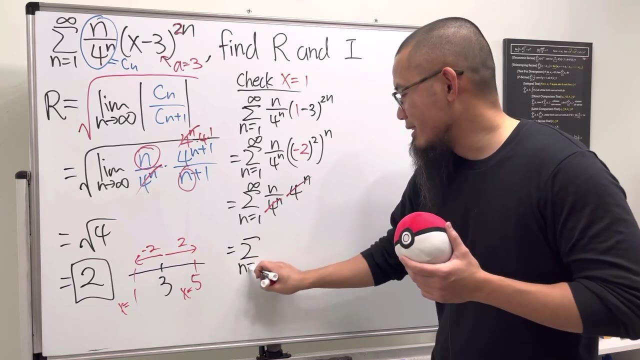 the series as n goes from 1 to infinity and we have n over 4 to the n. this is also 4 to the n and, as you can see, this and that cancel. so have a look. this is just the sum of all the natural numbers. n goes from 1 to infinity of n. 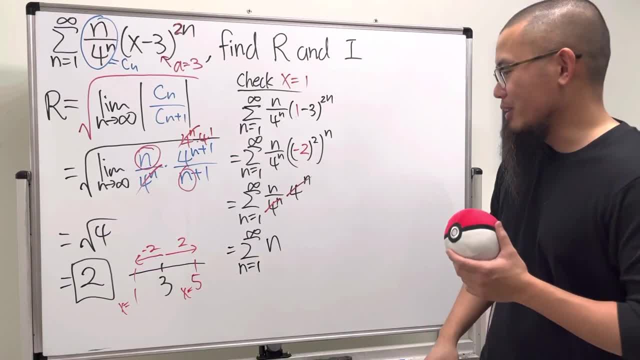 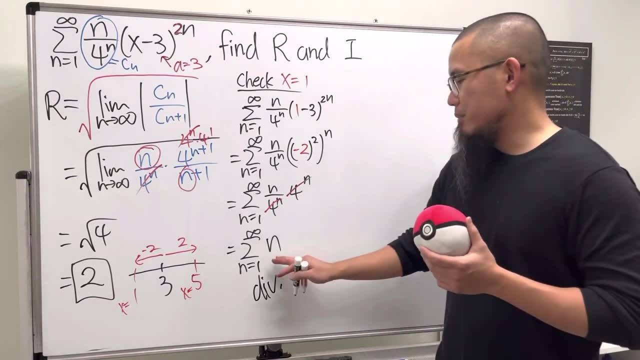 so it's just 1 plus 2 plus 3 plus dot, dot, dot, plus and so on. right, so of course this right here diverges. yeah, because you can use the test for divergence if you like, because this right here does not go to zero. all right. now the second. 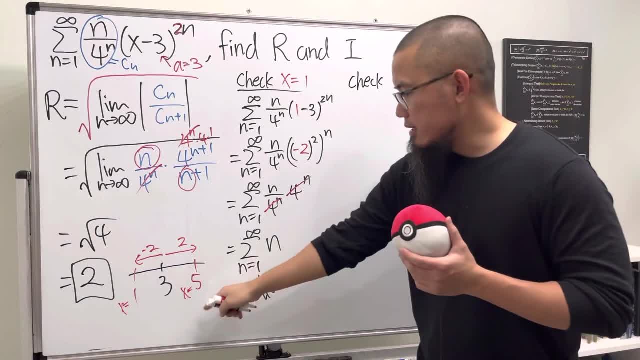 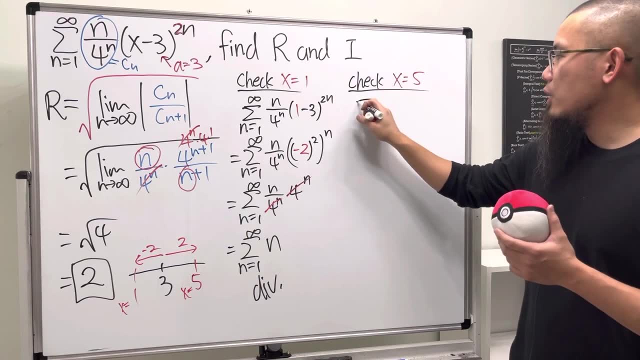 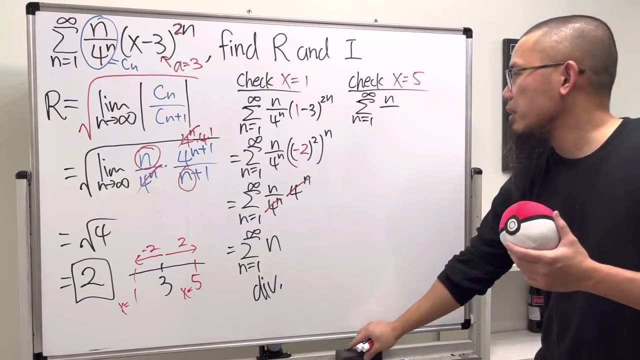 case is that we are going to check when x is equal to 5. all right, so pretty much do the same thing. plugging 5 into that x, we are getting the series as n goes from 1 to infinity and over 4 to the n, and then plugging 5. 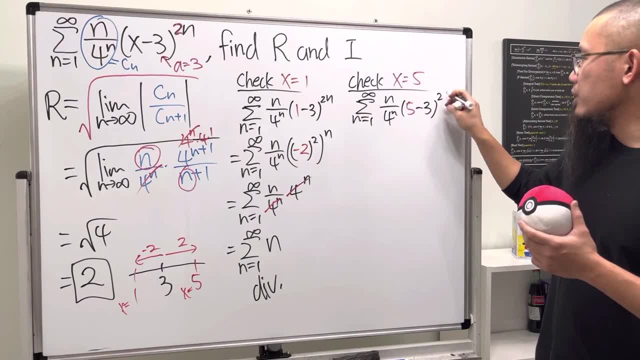 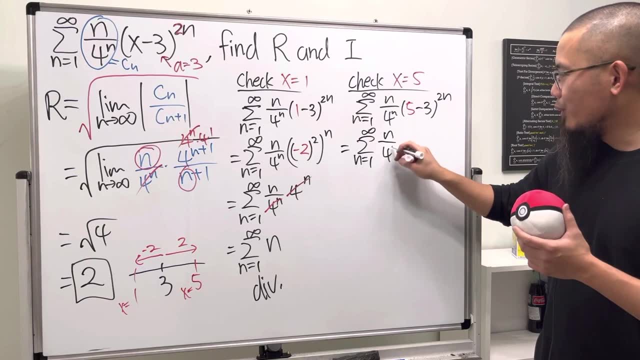 into the x and then minus 3, and then to the 2n power. okay, this right here it's the series as n goes from 1 to infinity and over 4 to the n. this is 2, and then we are going to do the same thing. 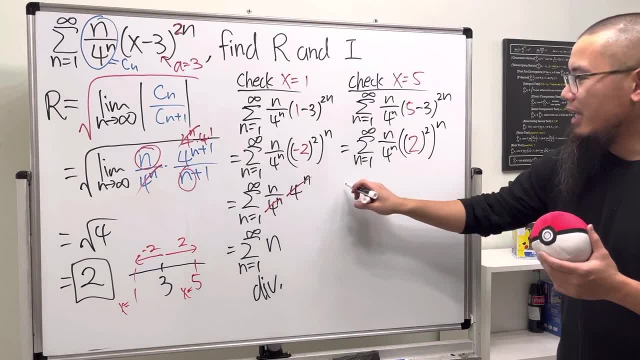 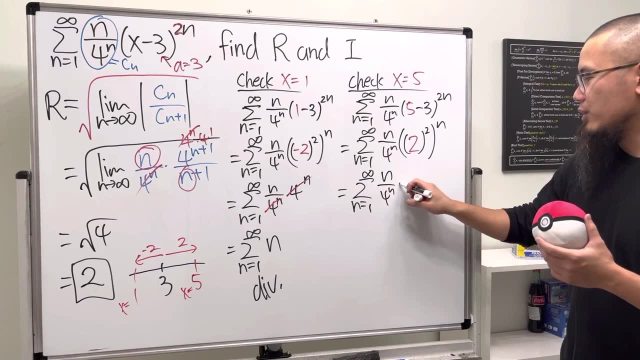 raise to the second power and then raise to the n's power and in fact we have the same situation and goes from 1 to infinity and over 4 to the n, and this is just 4 to the n as well. this and that cancel and we just